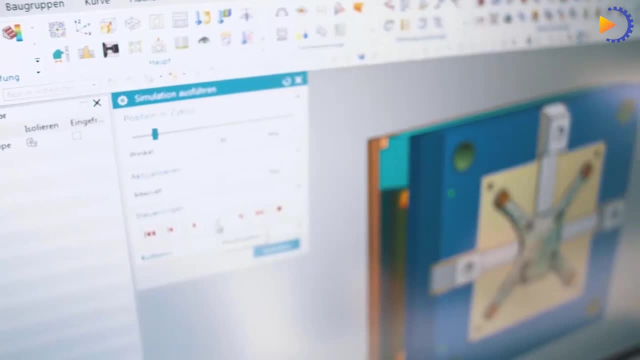 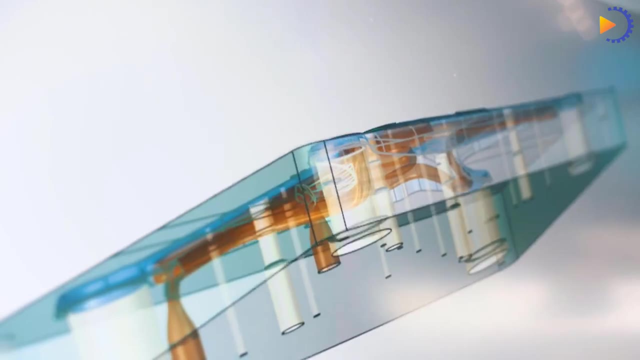 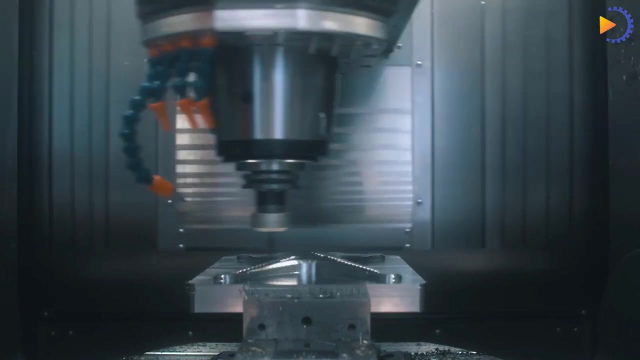 The CAME therefore aims to transform the geometry defined in the CADE software into a geometry understandable by the machine tool. Its purpose is to increase business productivity. Its use improves Adaptation to Market Needs. The quality of the products, thanks to the database. 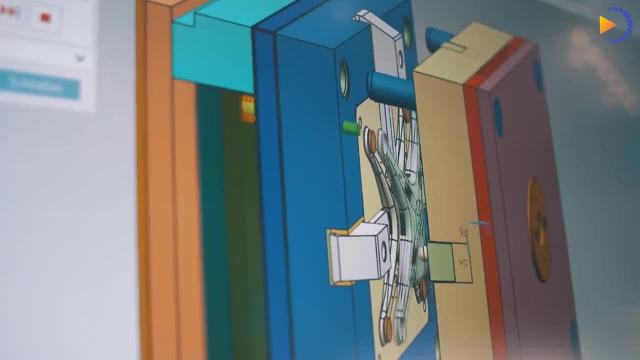 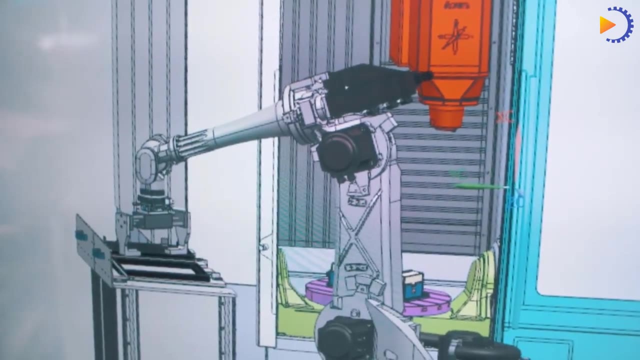 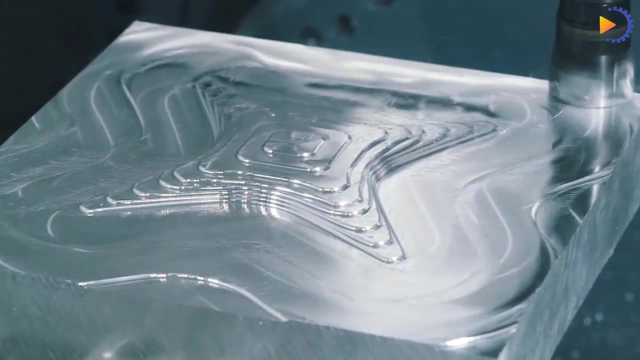 The database always accessible and updated regularly, and to the possibilities of simulating the trajectories on the screen. Productivity by the speed of obtaining an elaborate program Based on this definition. we need three components for a CAME system to work: Software that tells a machine how to make a product by generating toolpaths. 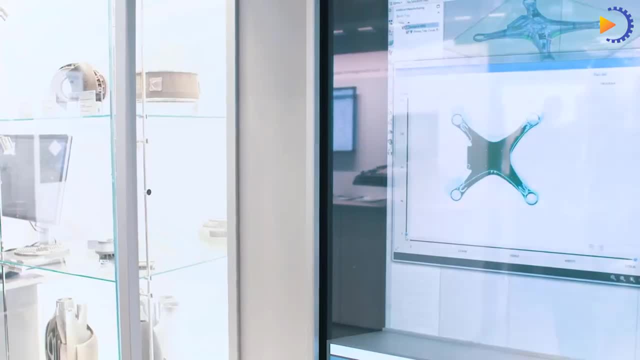 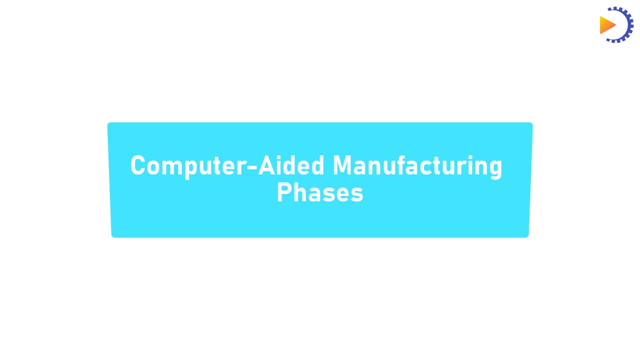 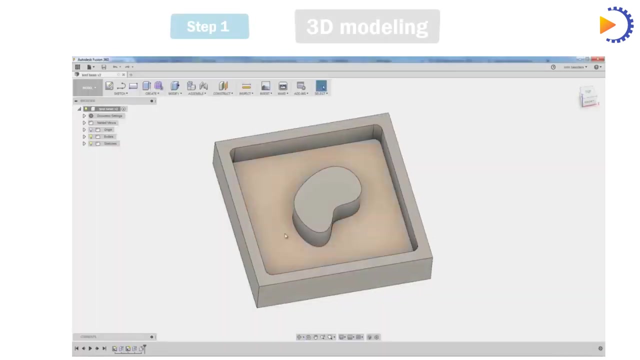 Machines capable of transforming the raw material into a finished product. Post-processing converts toolpaths into a language That machines can understand. The phases of Computer-Aided Manufacturing: 3D Modeling: The design of the part to be manufactured is carried out using computer-aided design CAME software. 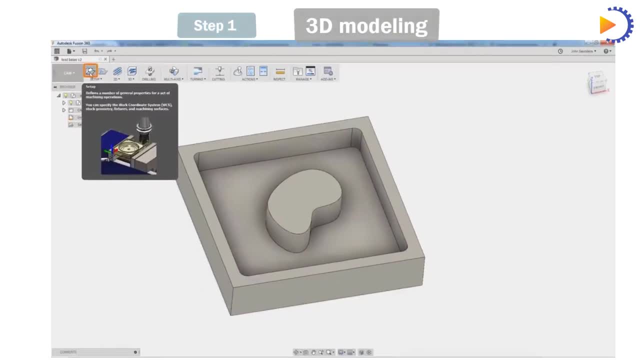 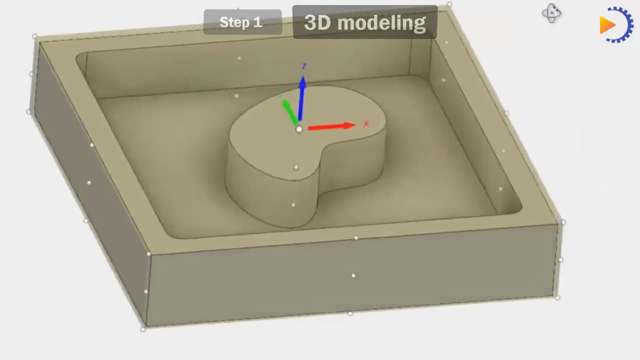 The file thus obtained is called 3D Modeling. This modeling is then exported, ie saved, from the CAME in an intermediate file using an exchange standard. In other cases, CADE and CAME are completely integrated. 3D Modeling. 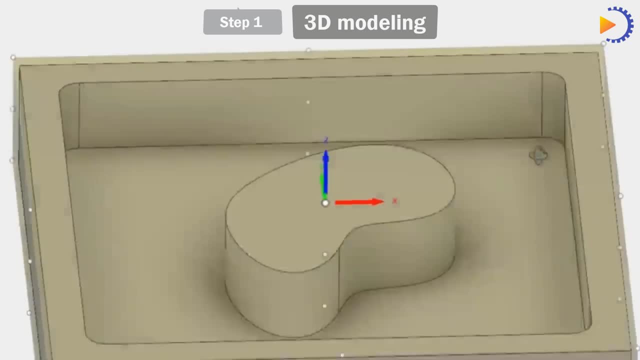 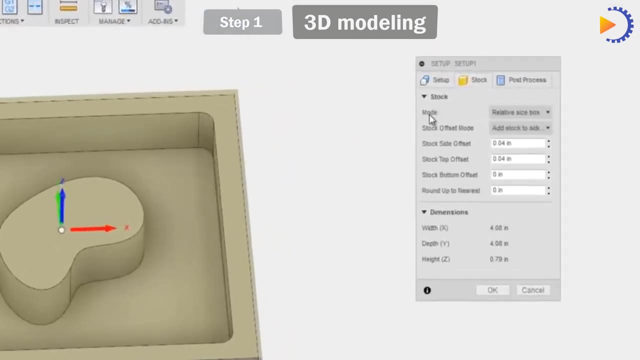 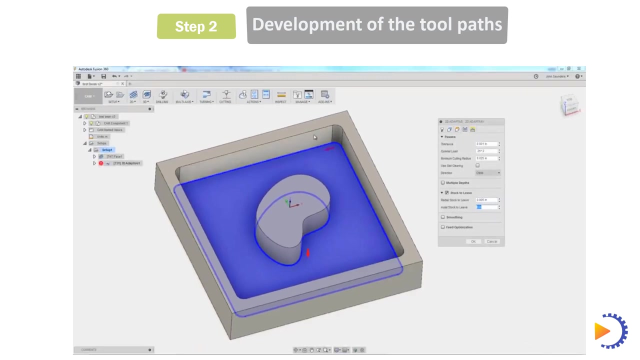 And do not require transfer. For these software packages. we speak of CADE, CAME, Such as CADEA and Fusion 360 software Software development After importing the 3D model into the CAME software package and then proofreading it. 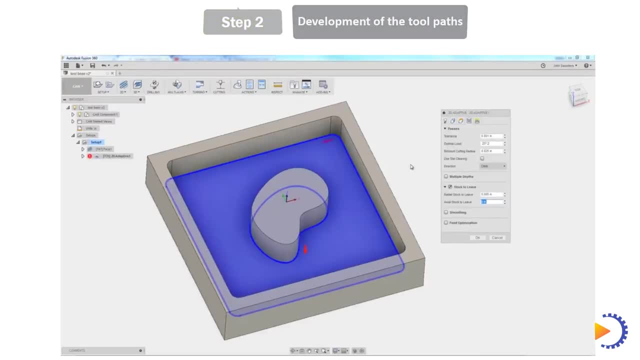 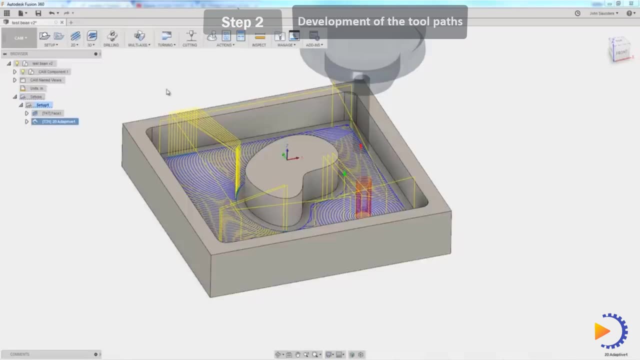 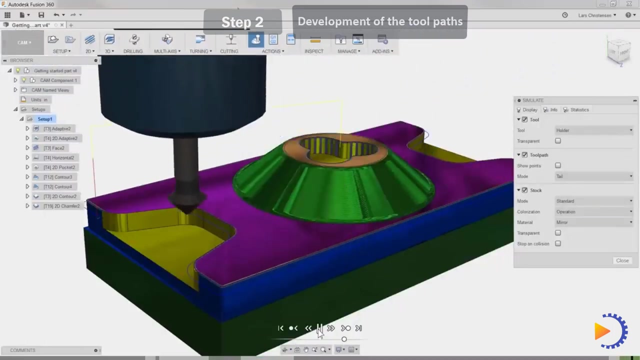 it is possible to move on to programming the toolpaths, which is the heart of the CAME activity. The programmer creates the paths while researching, expecting the tool choices, the cutting and feed rates and the machining strategies to be implemented, Then the simulation of the action of the tools and the material, thus allowing the 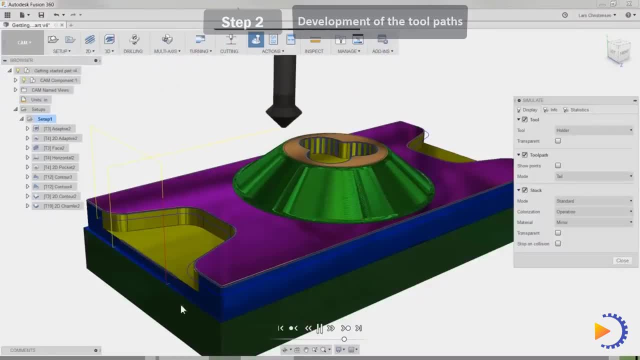 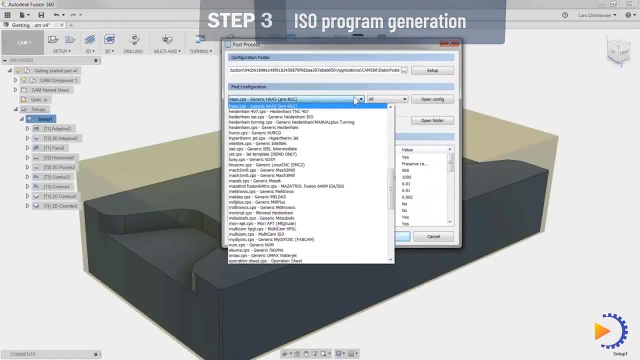 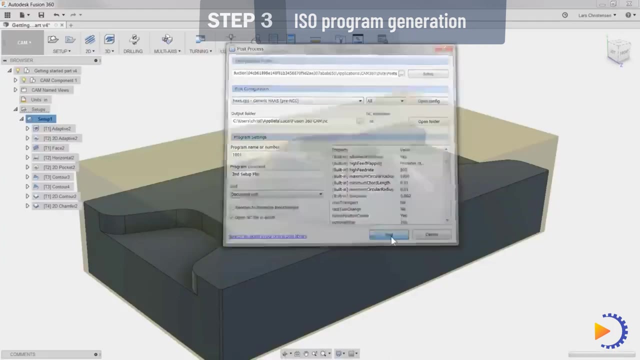 programmer to check his machining methods and to avoid a priori collisions on the machine tools. Generation of the numerical control program. The next step is from the CAME program developed to generate the ISO program used to drive the CNC machine tool, The program used for the conversion. 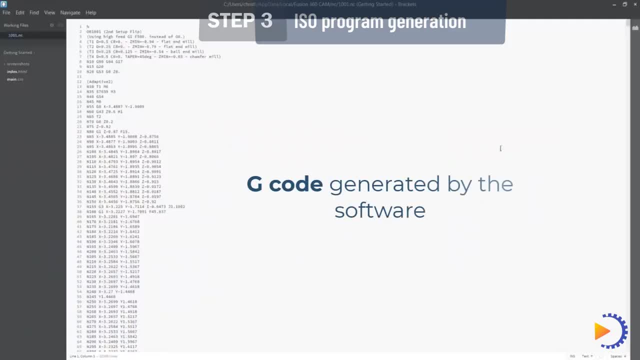 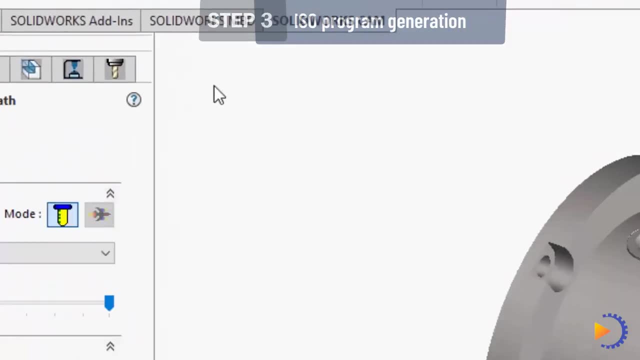 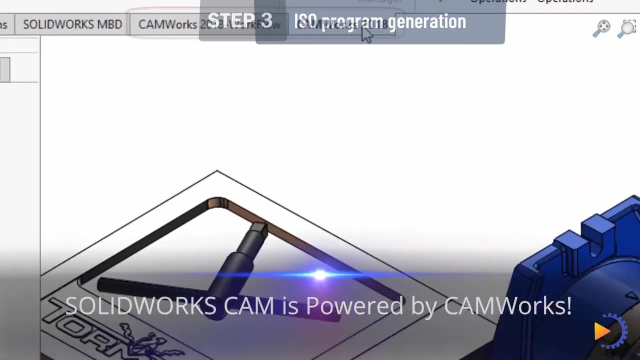 is called a post-processor. There are also independent machining simulation software programs that make it possible to reproduce the behavior of the machine tool in 3D by directly decoding the blocks generated by the post-processor. This makes it possible to take into account the 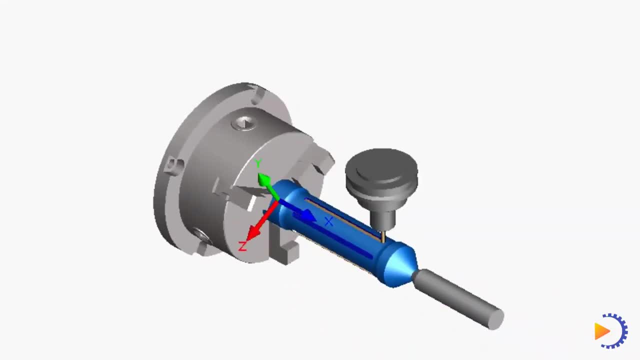 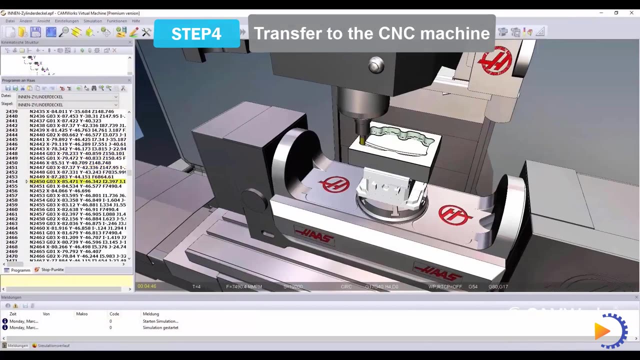 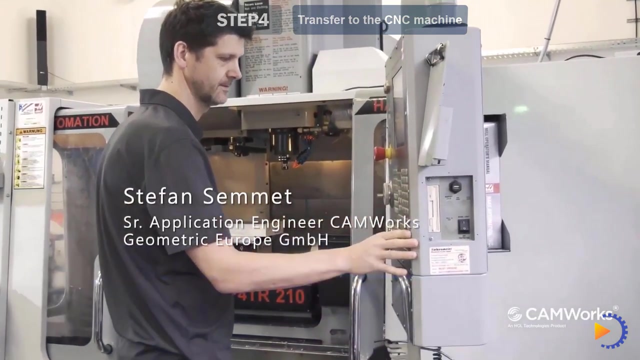 real program given to the machine tool and not the result of the CAME Transfer to the CNC machine tool. The ISO file obtained is transmitted to the MOC and numerical control program, A numerical control machine tool, by DNC direct numerical control software, then executed by this. 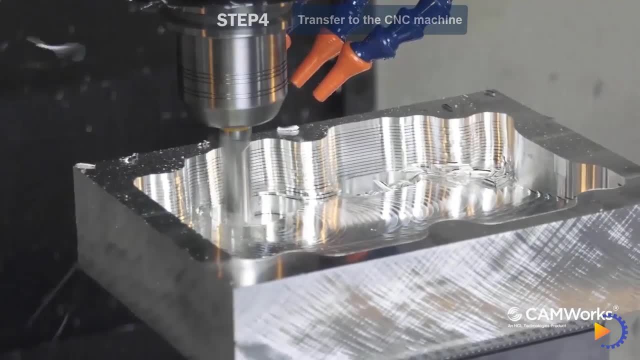 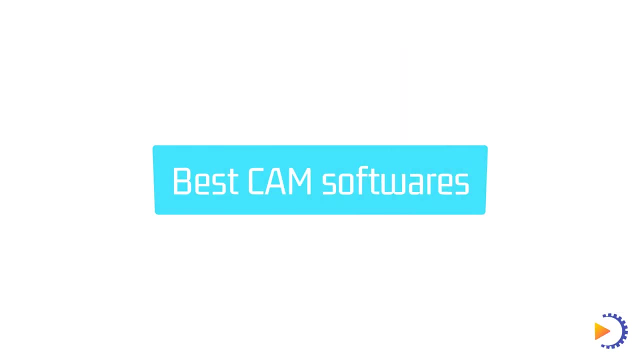 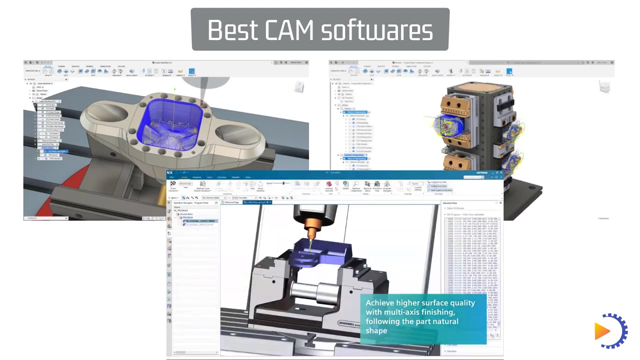 machine after the essential adjustment phase. A- numerically controlled machine tool. CNC is a machine tool equipped with a numerical control. Today there are a variety of CAME or CADE CAME software. Here are the top 10 computer rated manufacturing software One: 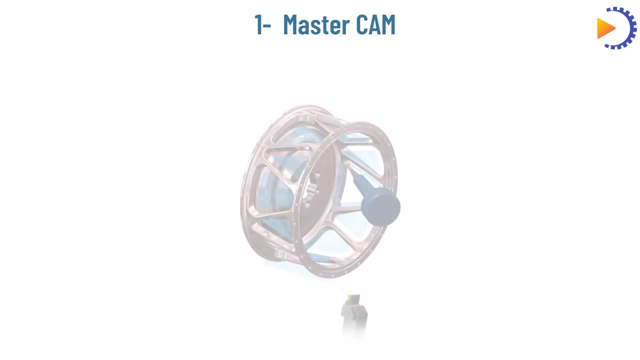 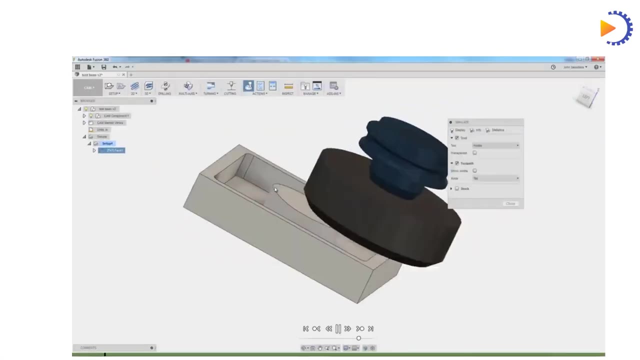 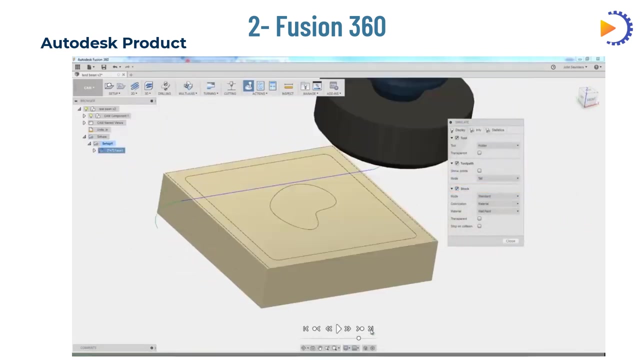 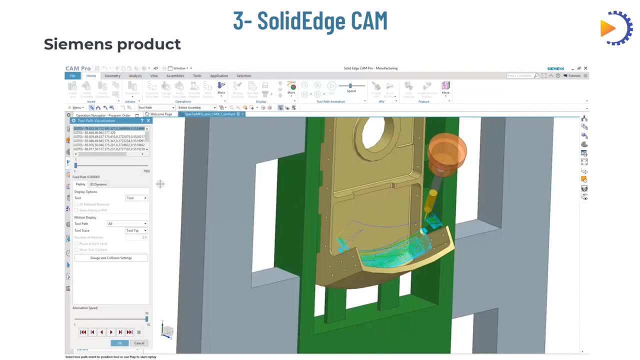 Master CAME. Master CAME software incorporates enhanced toolpaths and CADE tools. Two: Fusion 360.. Fusion 360 is one of the top 10 CAME software used in many manufacturing industries to develop the product. Three: Solid Edge. Solid Edge CAME software is the most widely used and easiest to use software. 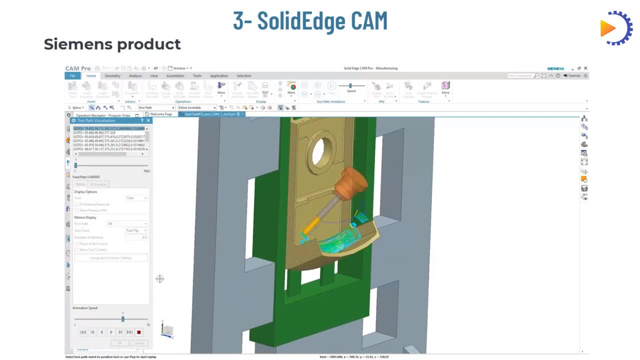 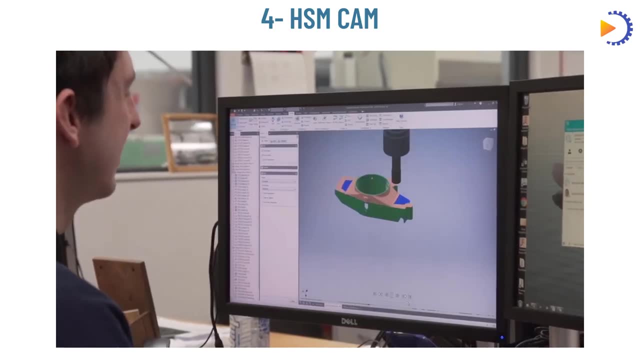 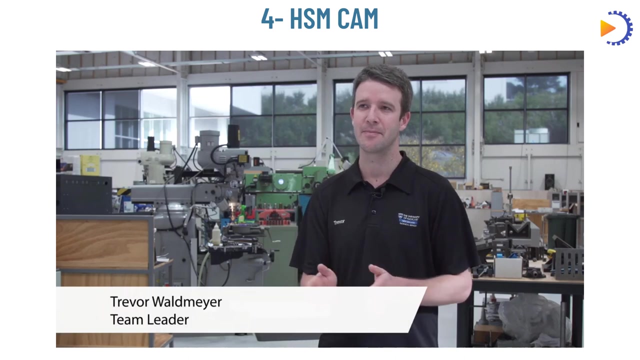 The main advantage of this software is that it performs all the operations of product development. Four HSM. HSM works. CAME software is the top 10 software used in manufacturing industries. The biggest advantage of using this software is that it reduces cycle time and has potential. 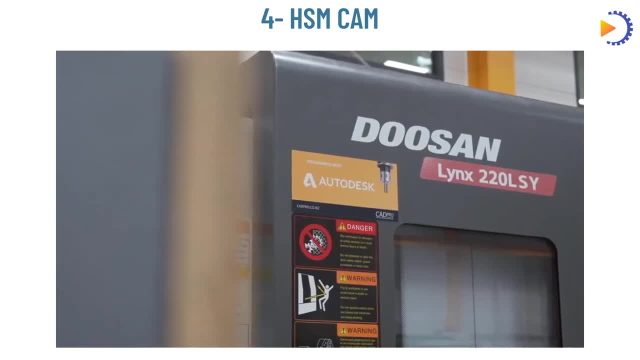 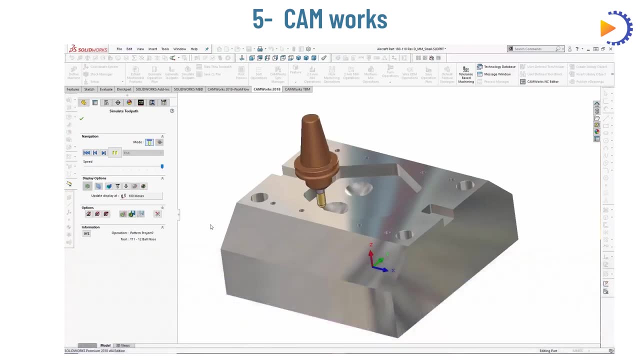 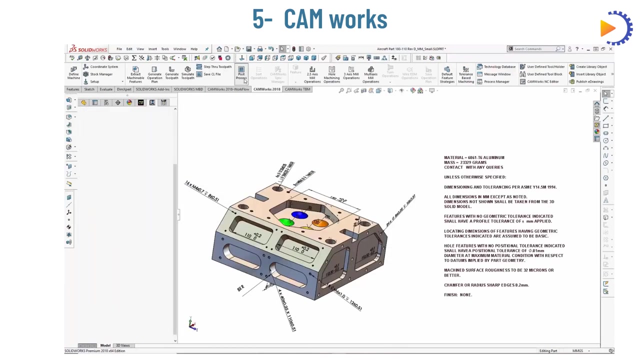 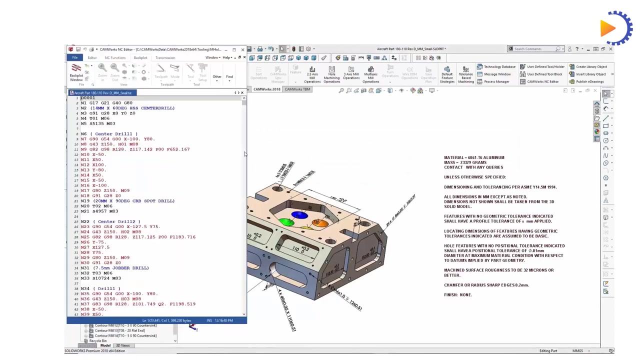 milling, turning and mill turn functionality. Six W HSE software. And what does the between Five? Solidworks, CAME. Solidworks CAME software is now integrated with Solidworks CADE software. The advantage of the software to integrate with Solidworks CADE is that it develops the product while it is in theoyre talking about CADE CAME software and not CAME. 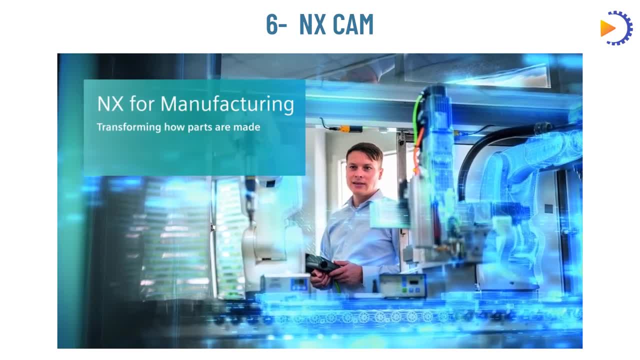 Six NX CAME. NX CAME software is the combination of NC programming capabilities and also manufacturer capabilities. The zero chrome programmes are forR Maker bit implement一定要. NX CAME software is the combination of NC programmingcom았어요 lenglikosoffware deciran, Top 5 of the myself.